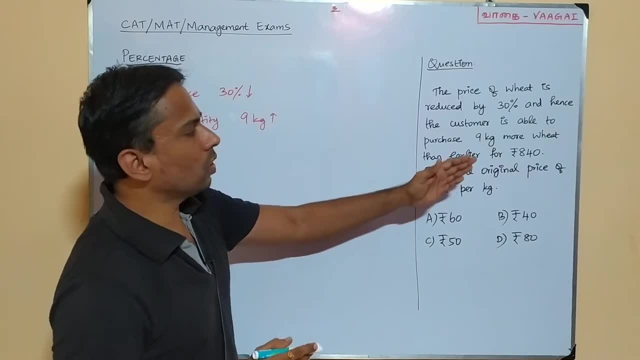 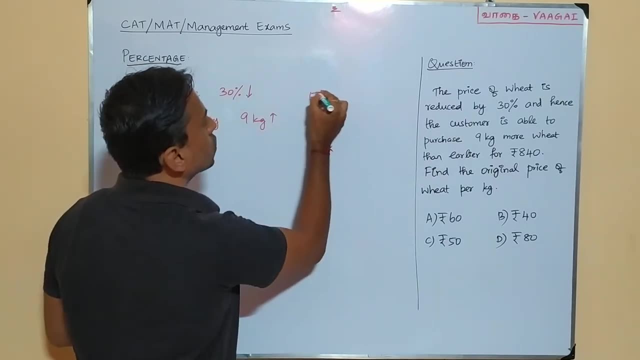 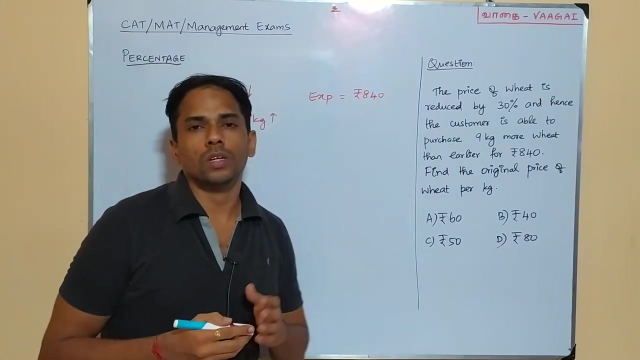 what is happening earlier than earlier For rupees 840- that is, the expenses- is what is at 840 rupees. So let's note down that also. So expenses is going to be rupees 840.. So the structure is going to be very simple. Price of. 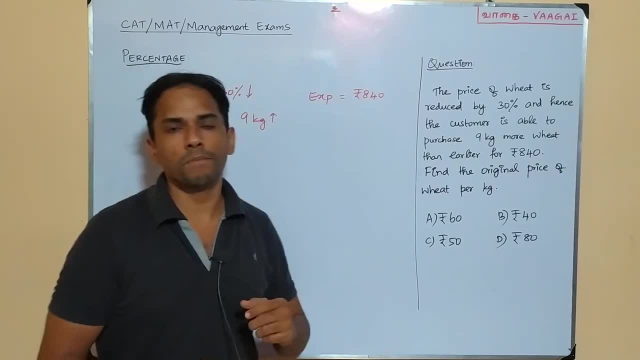 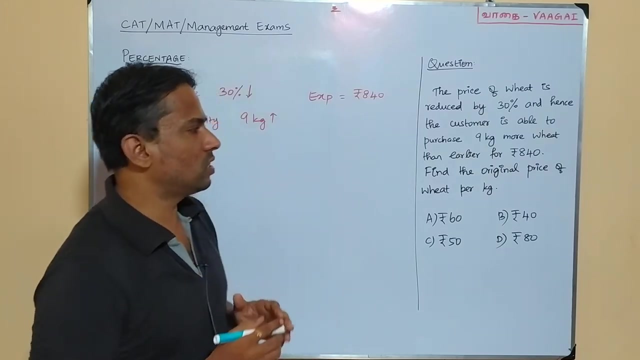 the wheat is going to reduce. it is going to reduce by 30 percentage and because of which, for a certain expense of rupees 840 rupees, the customer is able to purchase 9 kg more than the earlier stage. So that is what they are given. So if that is the case, then find what is the original. 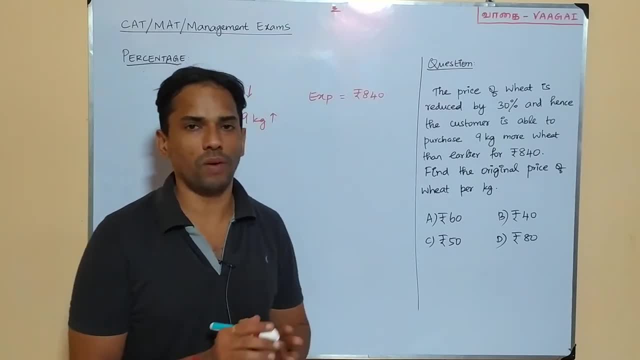 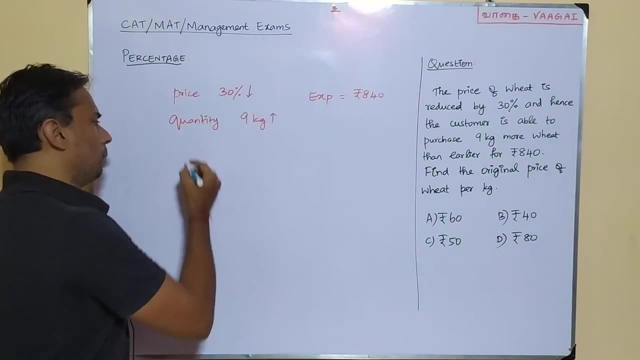 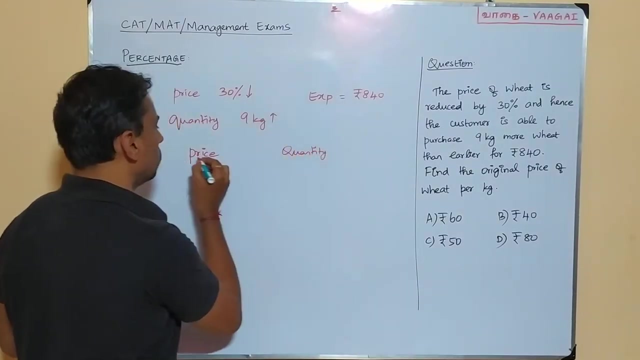 price of the wheat per kg. This is what we are asked to find Now. the setup is very clear for us. Let us now elaborate it. So they are just comparing price along with quantity. So that comparison is what is made here. So the price is going to decrease, and because of which 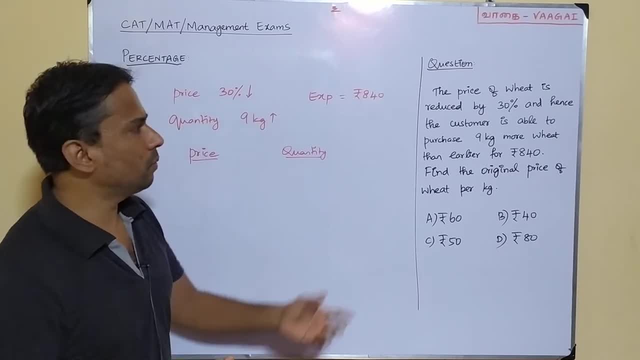 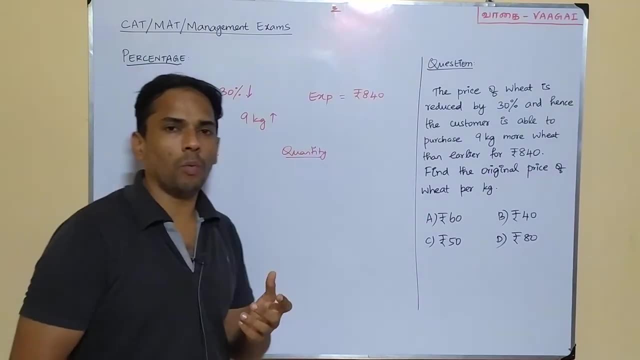 what happens? The quantity is going to increase. It is obvious, right? Because the expenses is kept constant here. in that case, When the price is going to reduce, what happens? The quantity, the amount of the quantity that we are going to buy, that weight that is going to increase only. 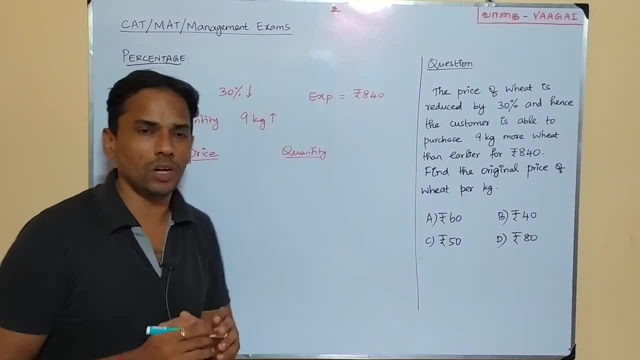 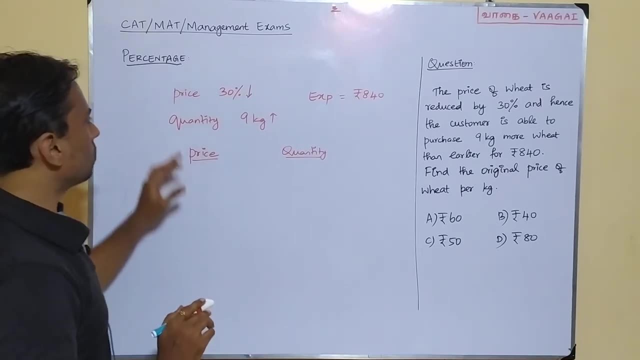 So they both are going to be actually inversely proportional, Is it or not? So let us, that is what I told. We will just elaborate the situation. So we will take some decent values here for our assumptions. So I am going to take it like price is going to reduce like 30 percentage. 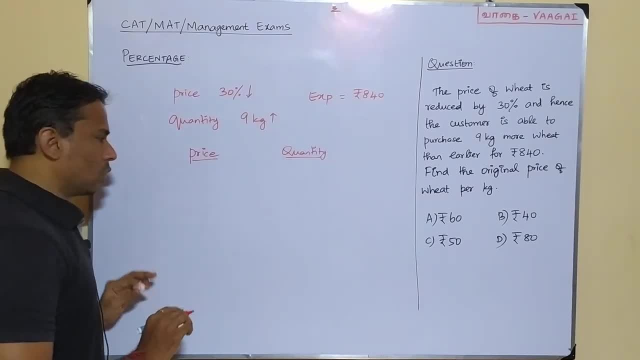 Price is going to reduce by 30 percentage. So what I am going to do is original situation. So let me write original here. and this one new situation. I am going to write new like this: So originally let us have it like some 100 percentage, So the price was like 100 percent. 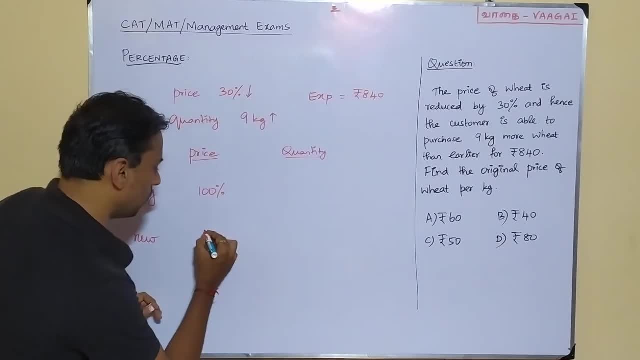 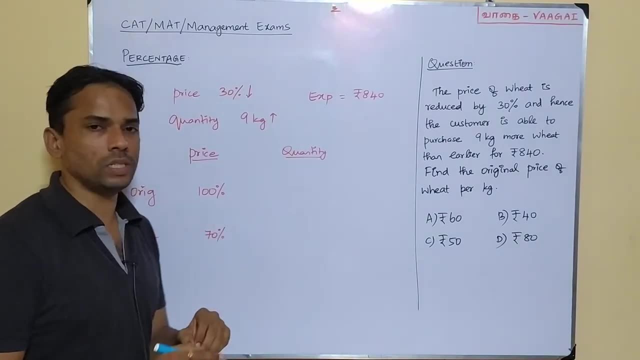 Now this is falling down by 30 percent, So that means the new price will be equal to some 70 percentage. So still, we are not having any idea about what is this original price or what is this new price. We are just comparing it with. 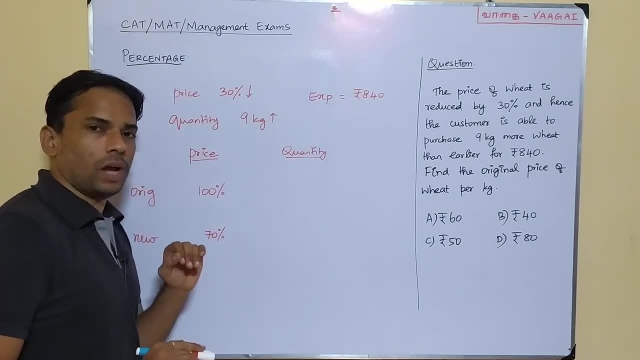 In terms of percentage itself. that is all, So original price. let us take it to be 100 percent. If that is the case, then that is the 30 percent decrease, right? So in that case, this new price. 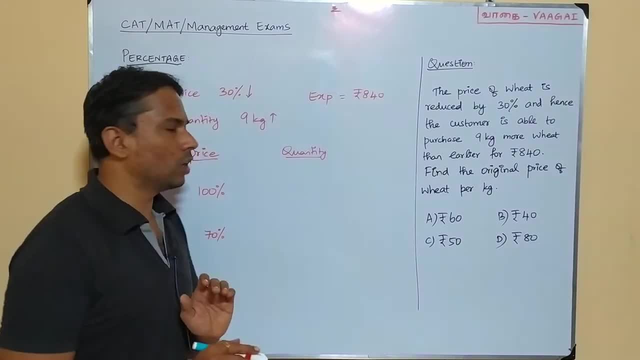 will become 70 percentage. Okay, Now come to the quantity here. Quantity also, they have compared. So what quantity originally that customer can purchase? now the customer is able to purchase 9 kg more, they have told. So here they have definitely compared in terms of kgs itself. 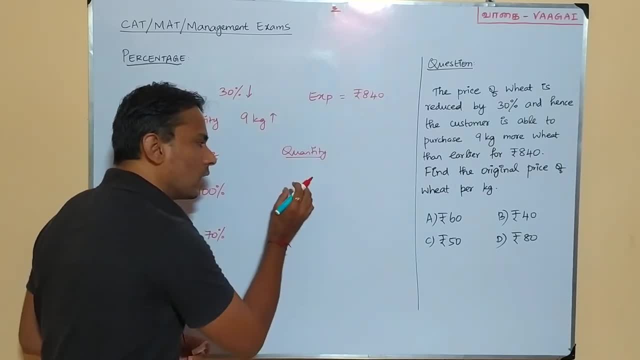 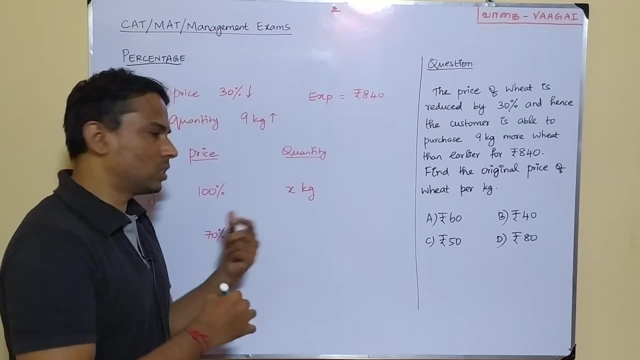 So in that case, here, what I am going to do is I am going to take the original quantity, The original quantity to be some x kg, So that the new quantity- I mean, like after this price reduction, the new quantity the customer can purchase. 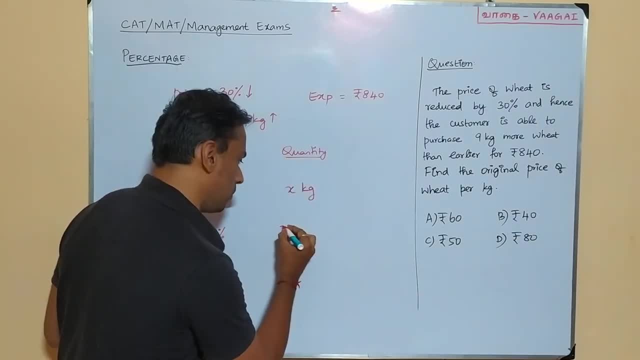 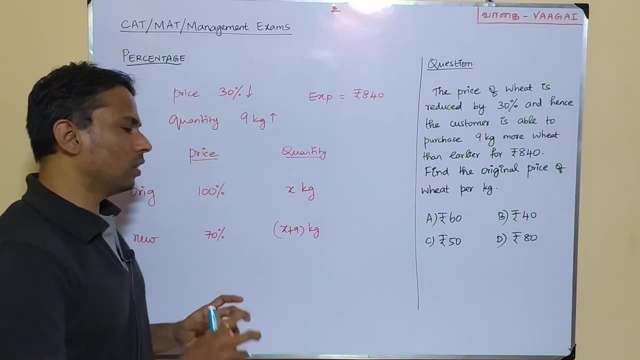 this will be nothing but 9 kg more they have given right. So that means this will be x plus 9 kg. So this is going to be our setup, right? Okay, Now hereafter we will just try to handle the. 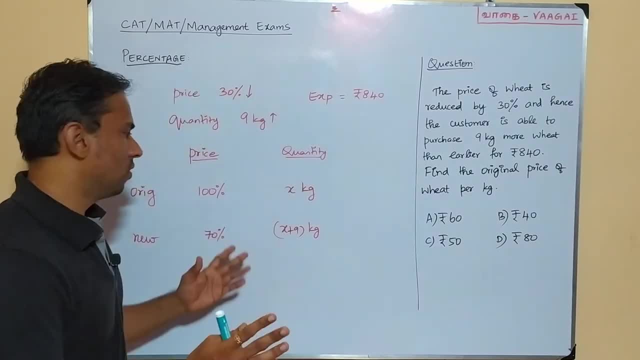 question in a smart way and then solve this problem. Okay, Yes, ready, Fine. Okay, Now price: it is going to decrease by 30 percent. We have taken 100 percent, 70 percent. What I am going to do is: 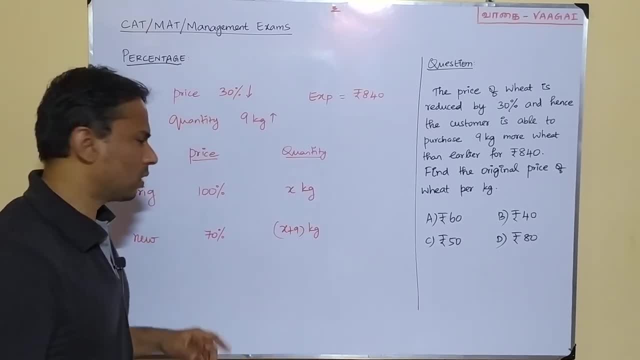 we are just going to take the ratio of the price. Ratio is going to be very simple, right, Because this is 100, this is 70. When you take the ratio, we will happen to get 10 is to 7 here. So remember it strongly. Price ratios are. I mean the ratio is to original, to new. that ratio is 10 is to 7.. Now price ratio is 10 is to 7. Since this price and quantity are inversely proportional. 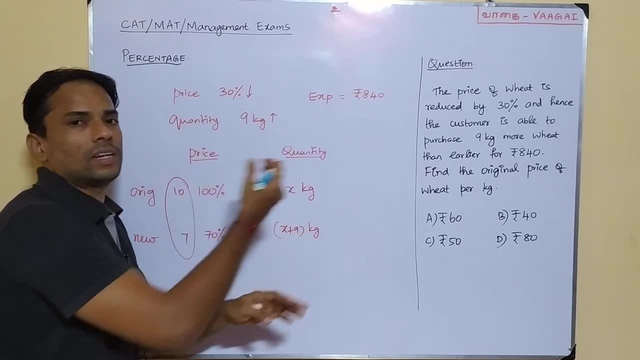 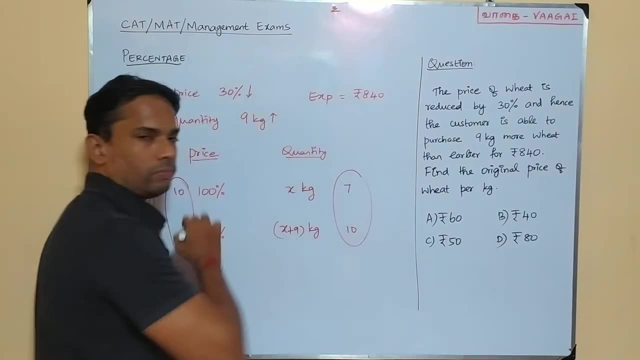 what happens to the ratio there. It will be exact inverse ratio there. So that means obviously quantity is going to be in the ratio 7 is to 10.. Let us note it here: Since it is 10 is to 7, there quantity is going to be, the ratio is going to be 7 is to 10.. 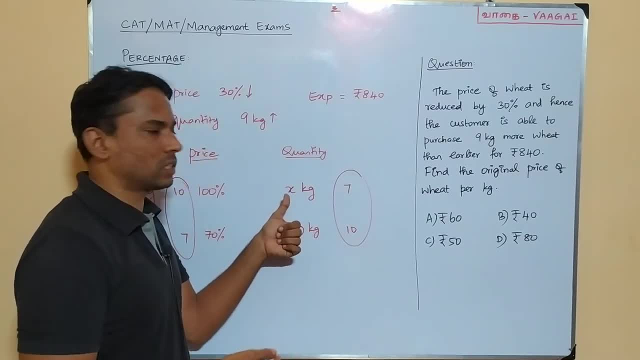 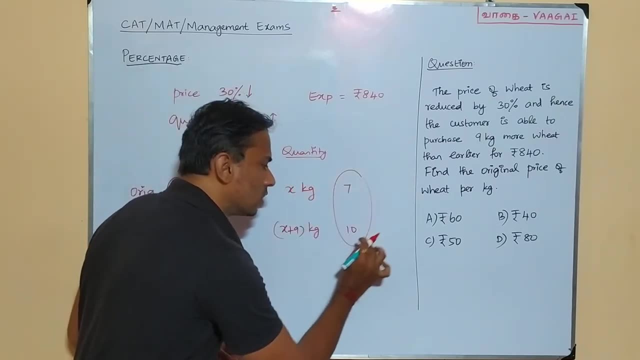 And this 7 is to 10 is what we have expressed in terms of x. This is like x kg and this is like x plus 9 kg. Or I can tell: this 7 parts is x kg, this 10 parts is like x plus 9 kg. 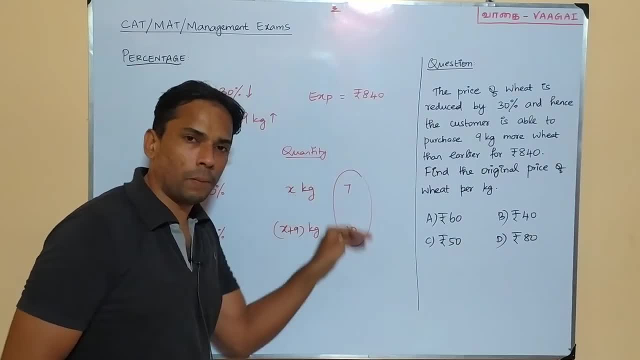 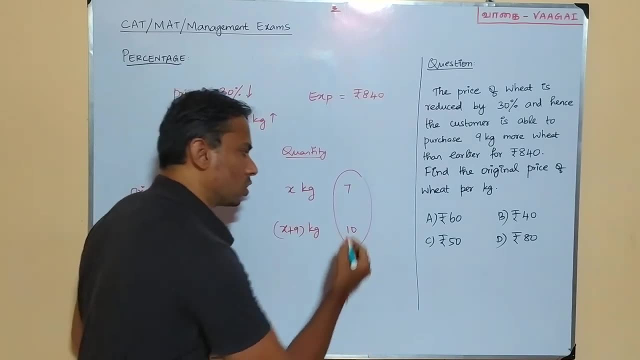 Now we have got 7 parts and 10 parts. here We will compare parts wise: this 7 and this 10.. This 10 is 3 parts more than this 7, is it or not? So strongly remember this 7 and 10 if you. 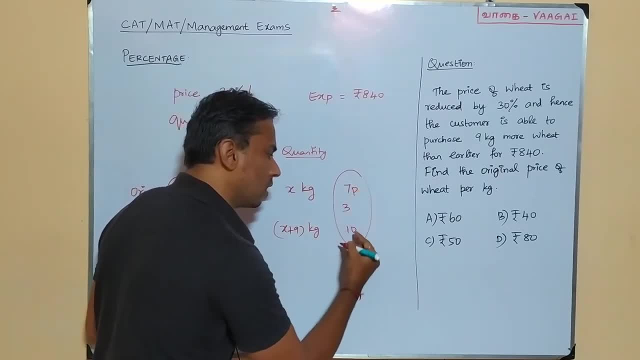 compare in terms of parts. if we compare this like 7 parts, this is like 10 parts. And how about this 10?? This 10 is 7 and compared to the 7, this is 3 more. So that means this is 3 parts more. 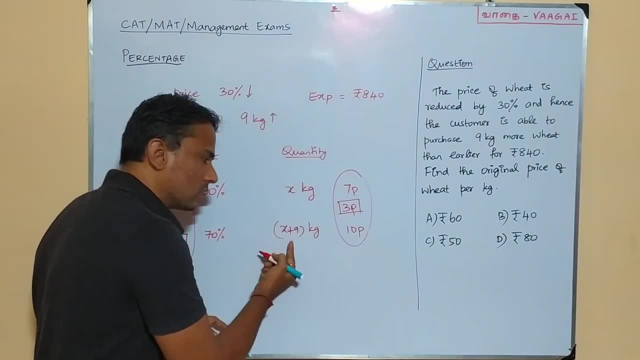 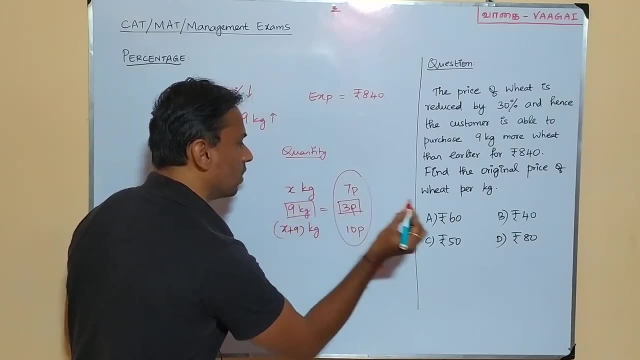 here And, kg wise, if I compare, this is x kg and this is x plus 9 kg. This is 9 kg, more right, So this is 9 kg. So we can very well compare, or we can very well. 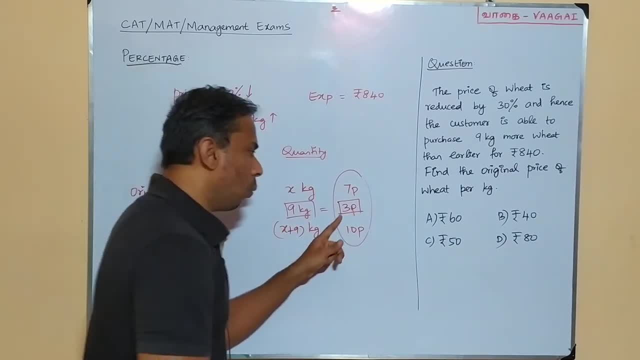 equate this: 3 parts is equal to 9 kg, So that means one part will be. so where can I use it? So I will use this space itself. This is enough. One part equal to 3 kg. So that means we can. 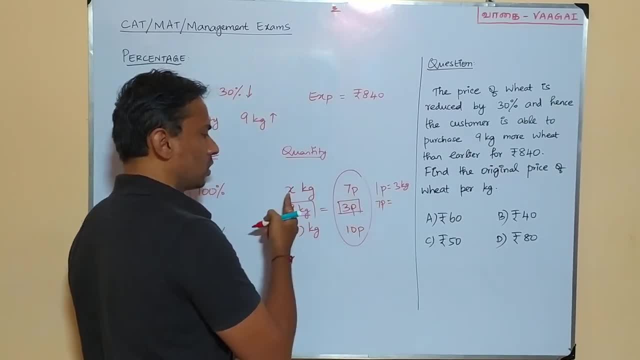 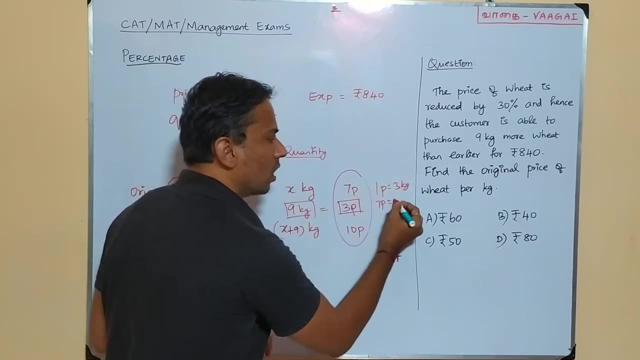 very easily get. 7 parts is equal to, because 7 parts is what is this? x, kg. So we can easily get the value of x. If one part is 3 kg, then 7 part will be obviously 7. threes are 21 kg. So 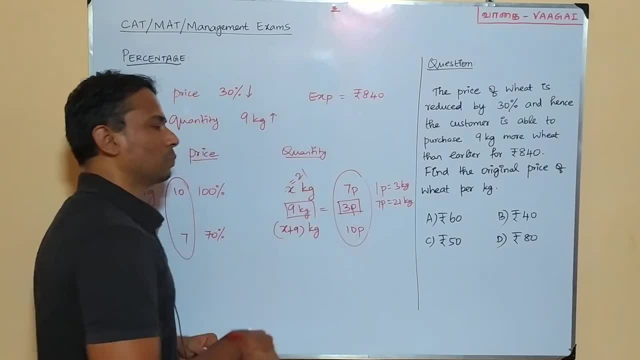 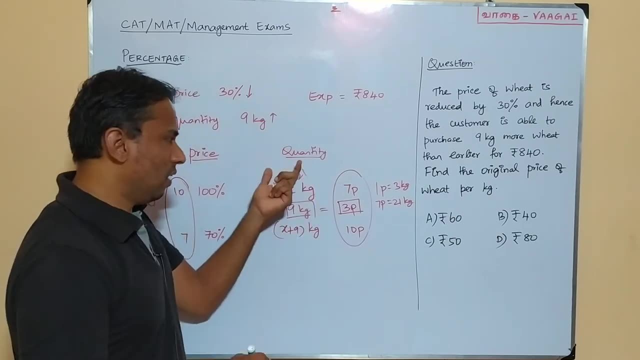 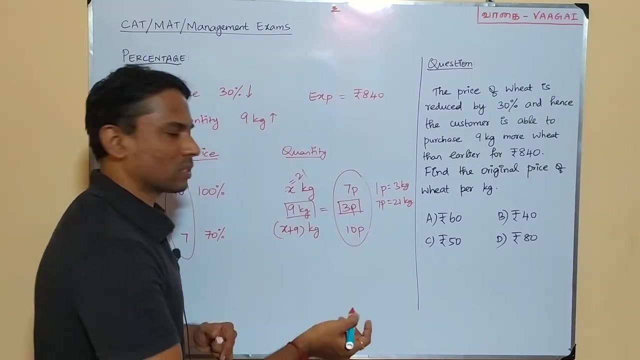 x value is going to be 21.. So I can replace now this x by 21.. So that means originally the customer is able to purchase how many kg- 21 kg- And after the price reduction now the customer is able to buy x plus 9.. That means how much? 21 plus 9.. So this will be equal to 30 kg. That's. 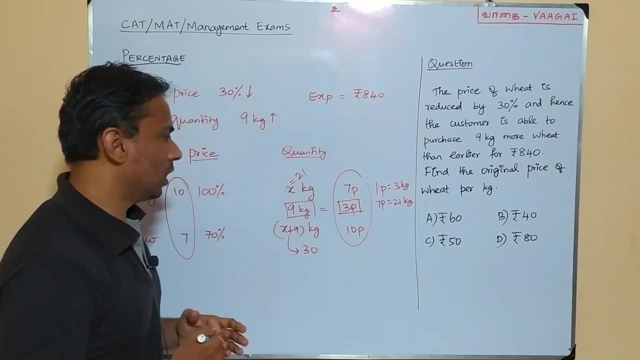 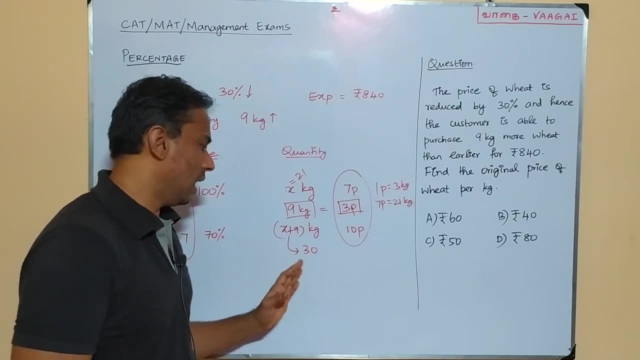 all. The situation is going to be very easier, right? Okay, So that means originally the customer was buying 21 kg. For what amount? For what expenses? 840 rupees, And now the customer is able to purchase 30 kg for the same 840 rupees. So 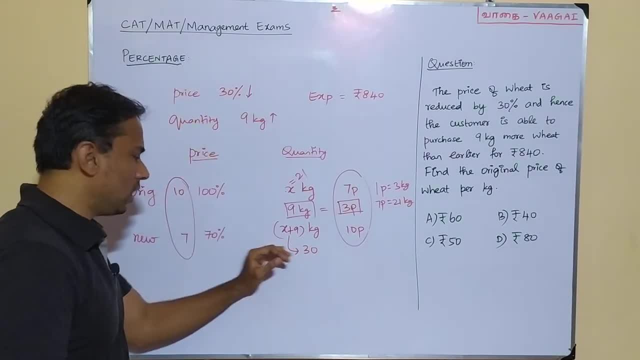 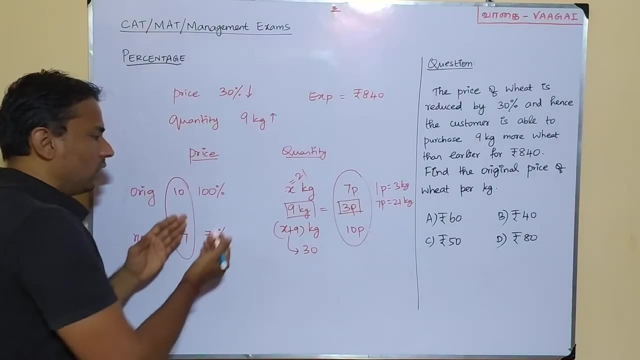 now we have got a clear idea about what is the original quantity and what is the new quantity. But in our question, what is asked here for us to find? We need to find the original price here. So so far we have assumed the price in terms of percentage only. But now, since we got that, 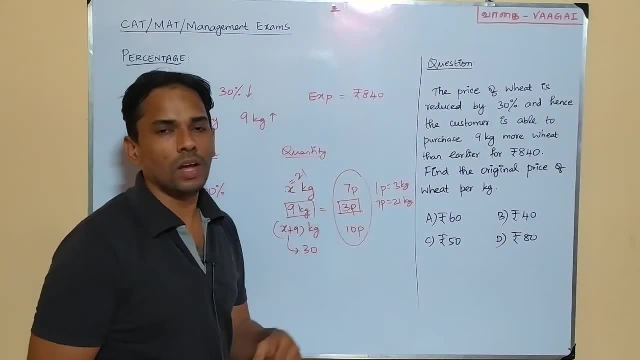 quantity. exact quantity x is equal to 21 kg. we got it. Now we can very easily get the answer. Fine, Yes, So how can we get it? It is very going, it is going to be very easy, So we can. 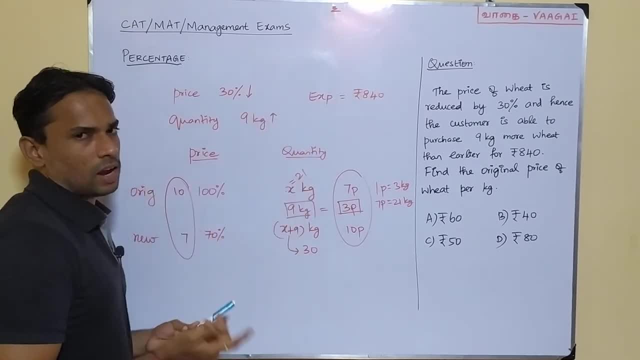 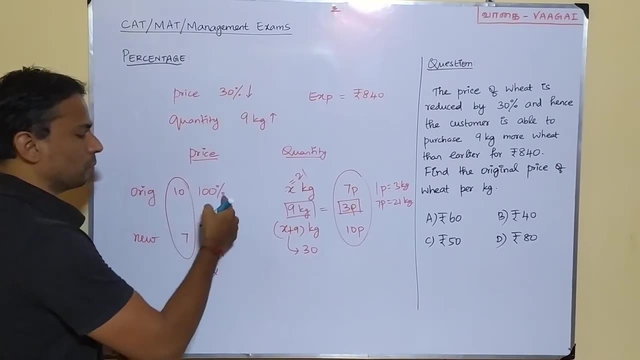 get it. So price into quantity is what is going to be, obviously 840 rupees. So in that case this original price, original price, will be nothing but price into. let me take it to be some P here. So price into this 21 is what is going to be, this 840 rupees. So I am going to take it as 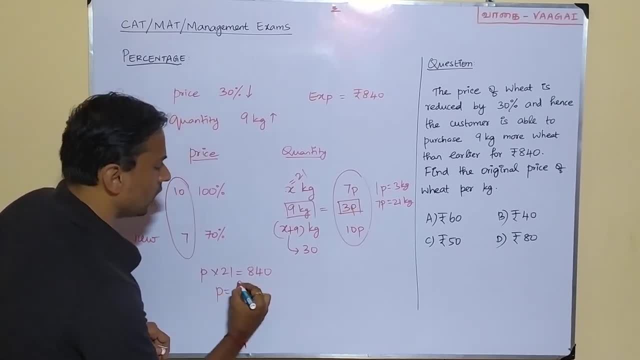 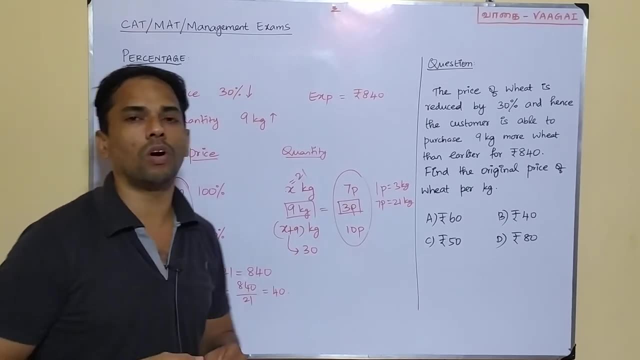 840.. So if you want to find the original price, this will be nothing but 840 by 21, and that is nothing but is exactly 4 times right, So 40.. So that means original price of weight is going to be. 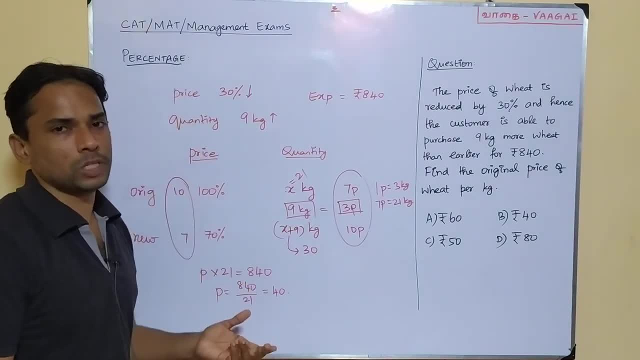 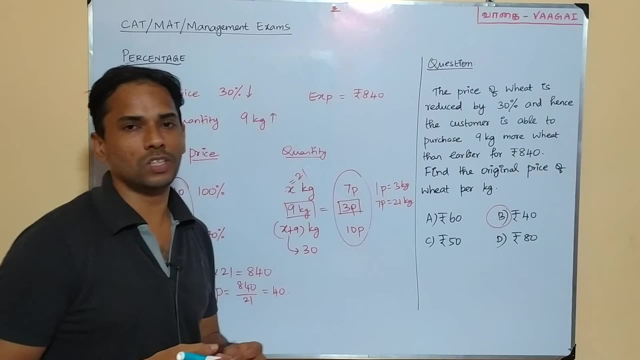 40 rupees. That is before reduction. it is going to be 40 rupees per kg and that's what you have, the answer. option b, option b 40 is going to be the answer for this question and again, if at all, suppose if they are. 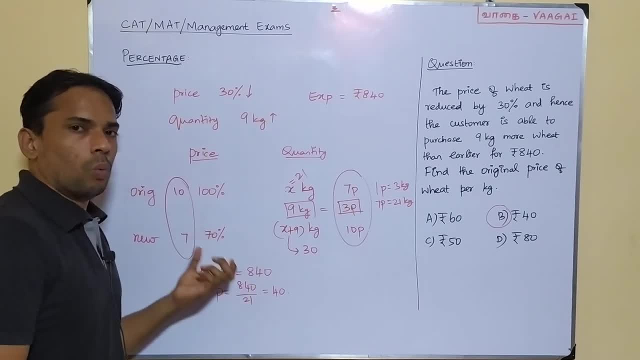 asking what would be the new price after reduction. what is the new price of wheat? if they are asking, it's going to be again simple. just one more step we need to do. we clearly know that the price is what the price is: 30 percent reduced, right? so we got the original price to be 40, right? so in that, 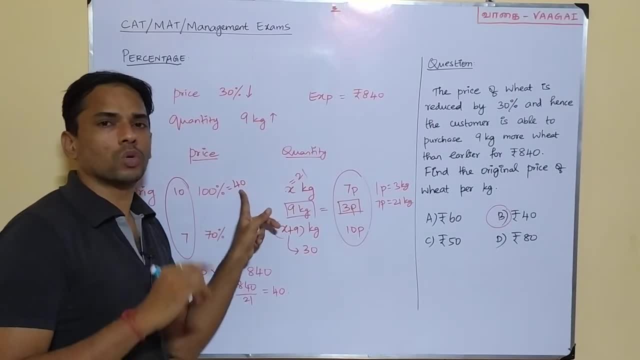 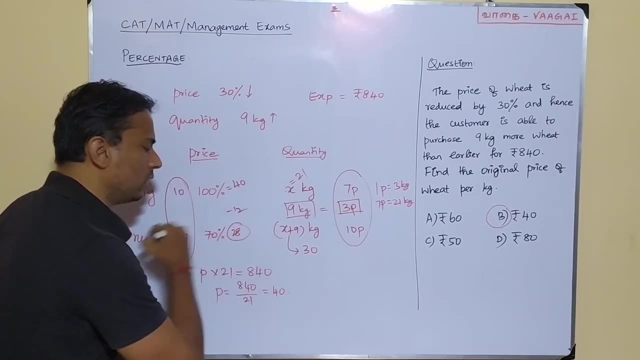 case we can take 40 here. what is 30 percent of 40? it is going to be 12, right? so that means this 40. we have to reduce by 12. so minus 12 we do, we get the new price to be 28. so that's it. so original price: 40. we calculate 30 percent of that minus 12, we do, we get 28 and that's going to be the new price of. i mean after reduction. the new price of wheat is going to be this only or otherwise. we can even use this ratios property right? okay, since we already have the ratio, this: 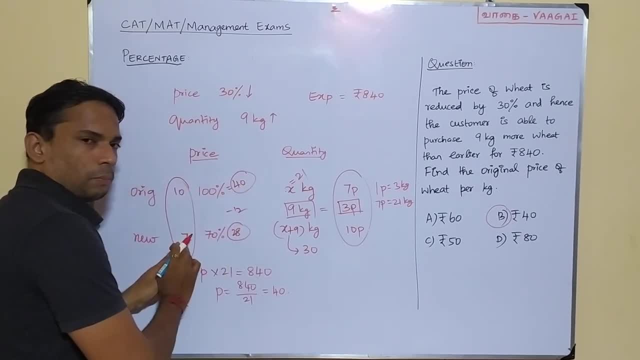 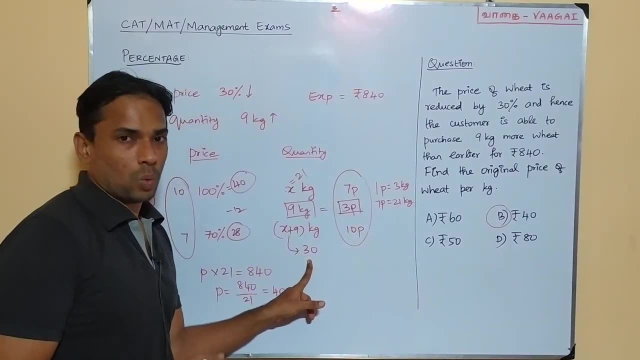 is 10 is to 7. this 10 parts is like 40. here again we can compare: 7 parts will be equal to 28. that way also we can get the answer or otherwise. however, we got the new quantity, also after reduction, how much we can buy the customer. 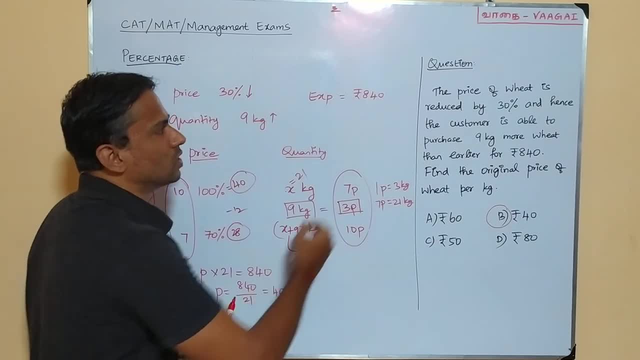 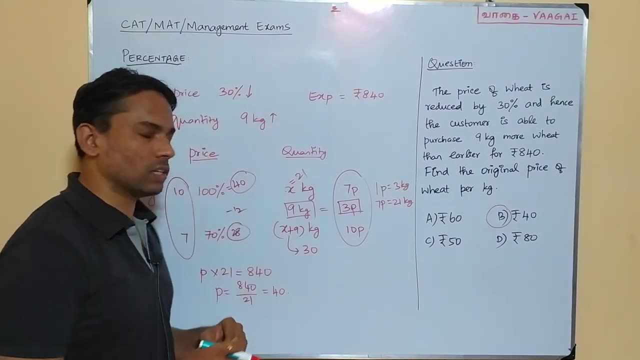 is able to buy 30 kg right. using that also, we can get the answer. just simply divide this 840 by 30. that will again give you the answer as 20, so there are many approach to get this, this answer also. but anyways, our question is asking what is the original price and for which the answer is 40. 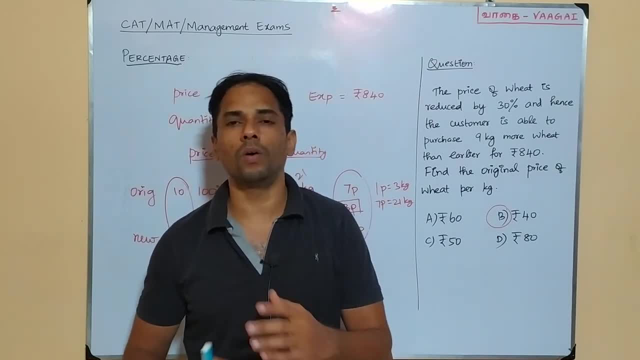 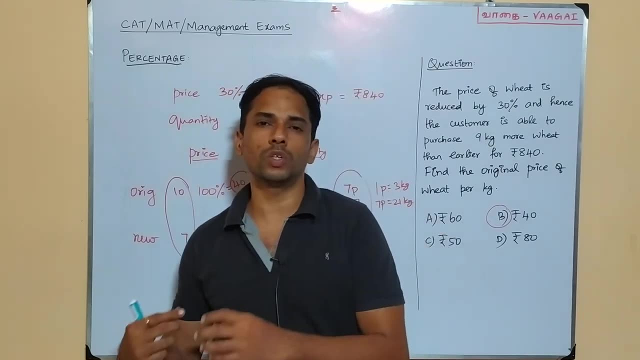 rupees per kg is going to be the answer. i hope you are clear with this problem: how we solved it, what steps we used it to solve it and everything is dear to you. so, without constructing any complicated equations, we just try to solve this problem using the properties of ratios itself. that's a objective of this problem. that's idea. 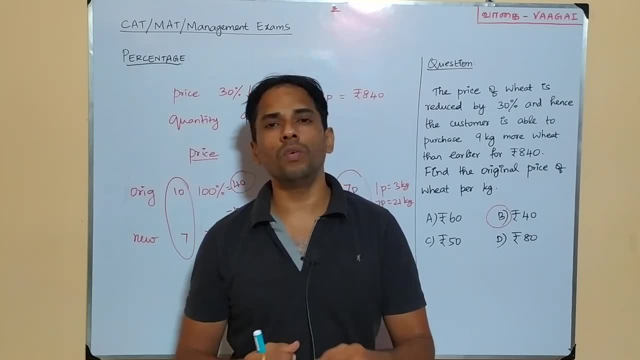 so i hope you are able to catch this. you are able to follow this. if you feel this session to be useful, please give a like, and if you feel that this session is going to be useful for any of your friends who are preparing for any such exams, please do share this video to your friends also. 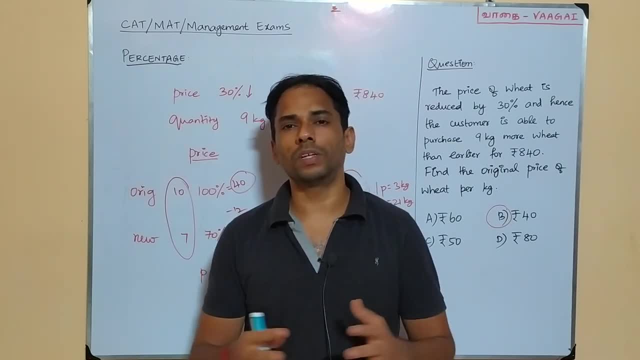 and again. we will soon catch up in the next session with some other interesting question. see you soon there. thank you so much.